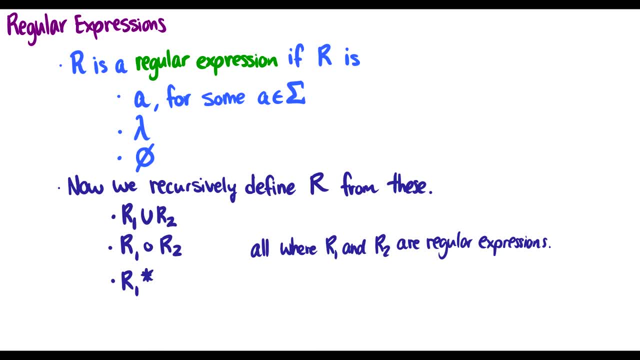 Welcome back to Mathematical Linguistics. In this video we'll talk about regular expressions. So before we've seen some languages that finite state machines accept. so instead of writing them out as sets with descriptions, we're going to write them as regular expressions. So r is a. 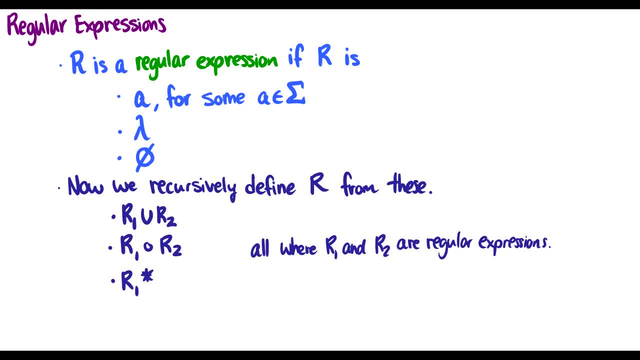 regular expression if r is either some symbol a for whatever a we have in our alphabet, the empty string, lambda or the empty set, And we can construct regular expressions from these three things recursively. So we can take the union of two regular expressions, we can concatenate two, 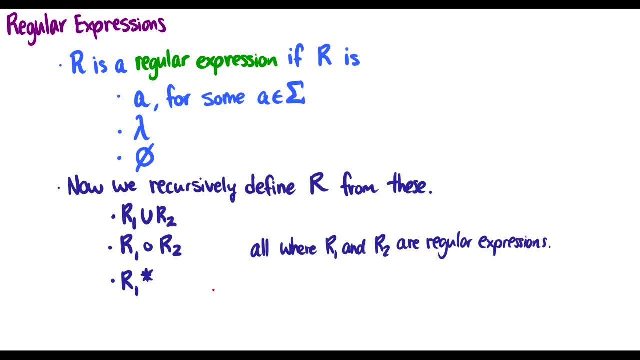 or we can take the star. So for instance, suppose we have r 1, which is just a, and we have r 2, which is b, Then we can concatenate them and we can get the regular expression a- b, or we get the regular 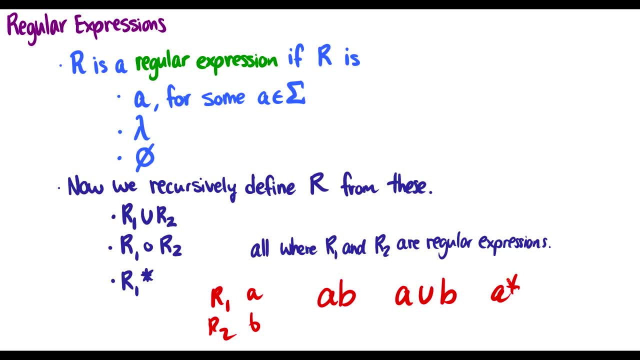 expression a union, b, Or we could get a star, b star, or a b bs, or we get a star, our plus a our亨, just A star. so we can really get whatever we want, as long as we follow one of these three rules. 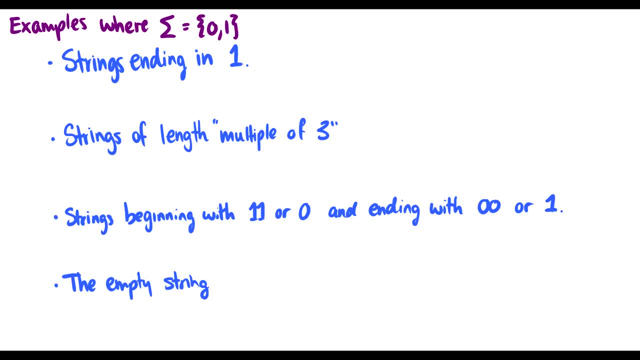 Okay. so let's write these languages, which can all be finite state machines, as regular expressions. So the first one strings ending in 1.. So we have an alphabet just 0 and 1, but we know that the final thing we want is going to be a 1,, so let's end this. 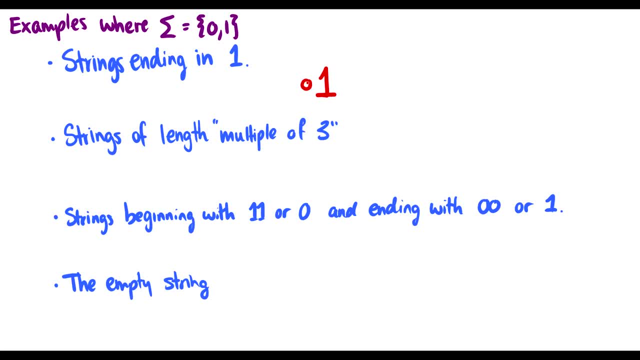 with a 1.. So we're going to have something concatenated with 1,, but really it can be any string, so it could be 0 0, 0, 0, 0 ending with a 1, it could be 1 0, 1 0, 1, 0 ending with a 1,. 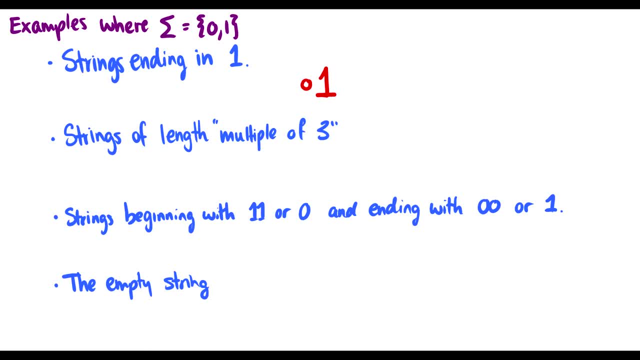 it could just be the empty set, then ending with a 1,. so really we have E star or sigma star here, So we can take any number of zeros and ones and then we concatenate it with a 1, and then that is the string's ending. 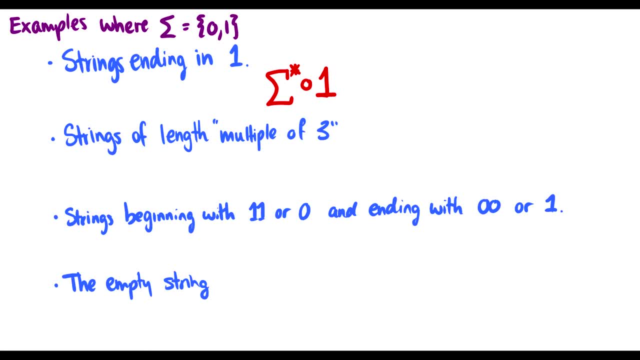 In one regular expression. so usually I don't put the concatenation symbol in there. so if I have sigma star 1, this just means any amount of sigmas or any amount of symbols, and then just a 1.. Okay, strings of length multiple of 3.. So we want say 0, 3, 6, 9, 12,. 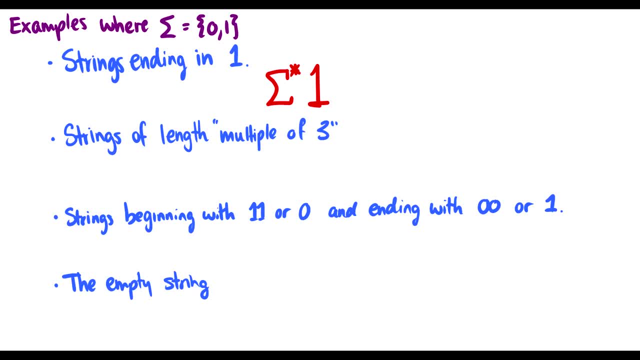 we want strings of that number. So what we can do is we can say: okay, well, if we just take three symbols and then we put a star here, this will produce strings that are either 0 symbols long, 3 symbols long, 6 symbols long, 9 symbols long. so the star operates on the 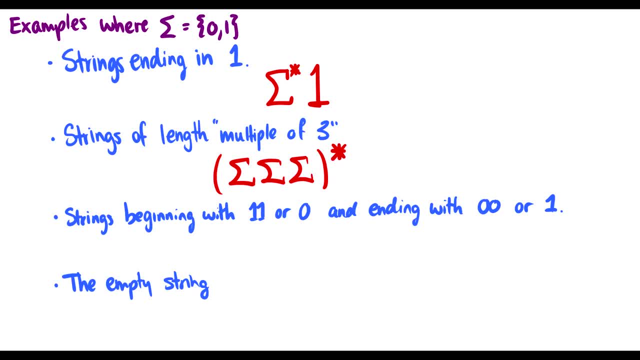 whole parentheses here. Okay, so if we have multiple of 4, so let's say this was 4, then we just add another one, and then we'd star it. so now we'd only get multiple of 4 here. Okay, so that's the star concatenation operator, So strings beginning with 1, 1 or 0 and. 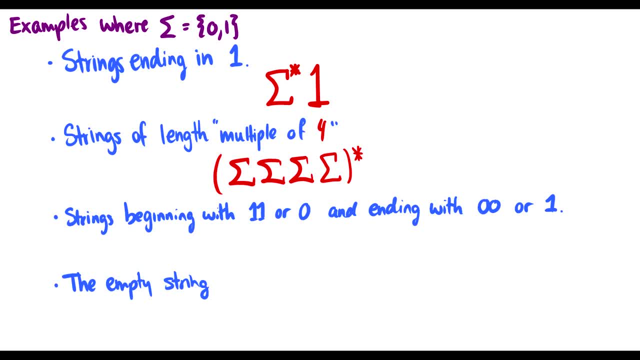 ending with 0, 0 or 1.. Okay, so here's where we introduce unions. So it begins with 1, 1 or 0, which means we can have a 1: 1 union, 0, so this means we pick one of these in this step. 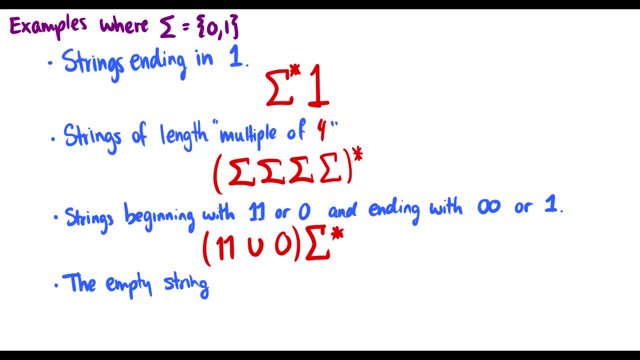 then we can have anything in between. so we have sigma star in between, and then it ends with 0, 0 or 1, 1, so it ends with either 0 or 1.. So that's the star concatenation operator. So strings beginning. 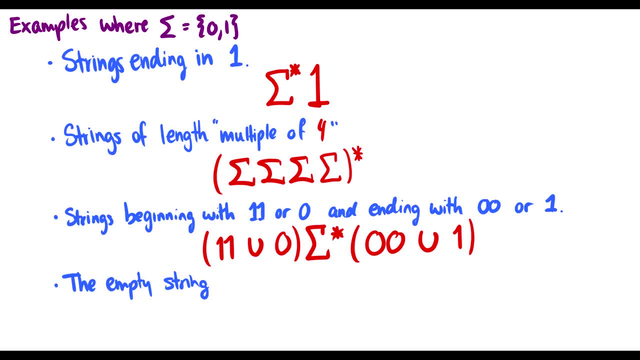 with 0, 0, 0 or 1, 1.. So what this means is: first it takes symbols out of our first bit, it does any number from sigma star, and then it picks from either 0, 0 or 1.. So this follows the. 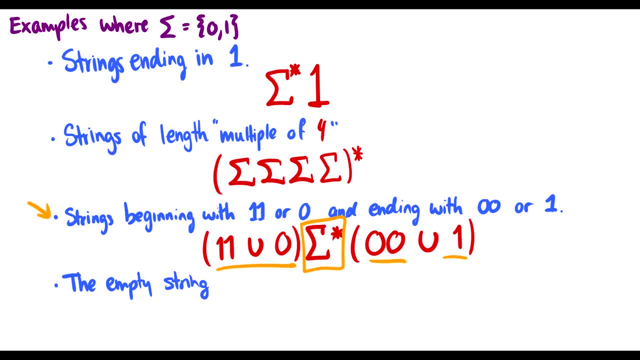 guidelines here. And finally, the empty string. So we could just say, okay, this is lambda. or we could say that this is the empty set star. So remember, if we take the star then we'll always get the empty string out of it. but the empty set has no symbols in it. 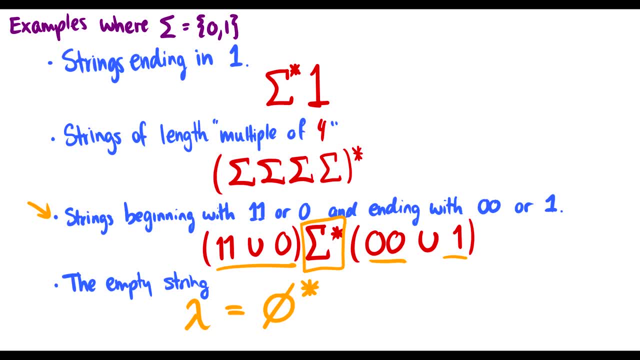 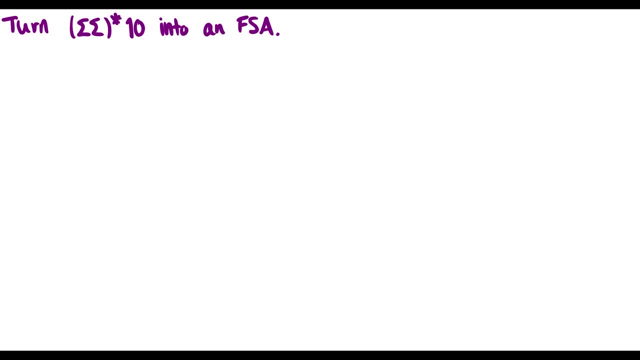 So when we take the empty set star, it's just equal to the empty string. Okay, so those are some examples. So let's turn one of these regular expressions into a finite state machine. Okay, so I've already showed this conversion before with languages, but now we can do it with symbols. So 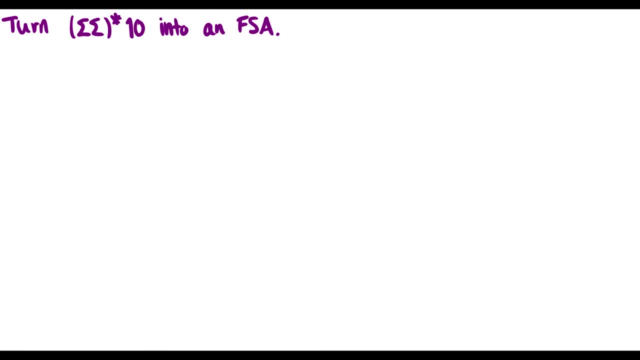 here's what we do. So there's really a lot of concatenation going on here. I just haven't written the concatenation in. So, for instance, let's rewrite this concatenated, So we have sigma concatenated with sigma, we've taken the star of this, then we concatenate it with a 1, and we concatenate it with a 0.. 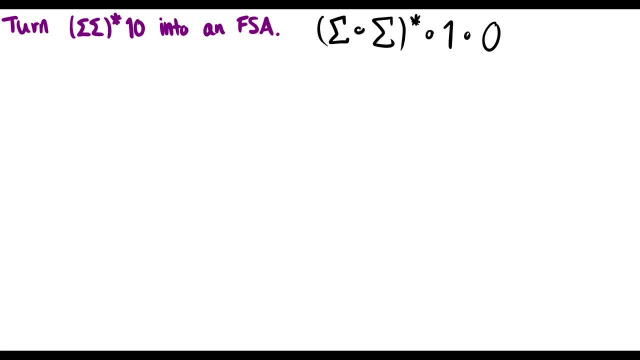 So we can write finite state machines for all of these. So, for instance, the first sigma here is going to have a start state and it's going to send 1 or 0 to the end state. So this is the first sigma. Then we have our second. 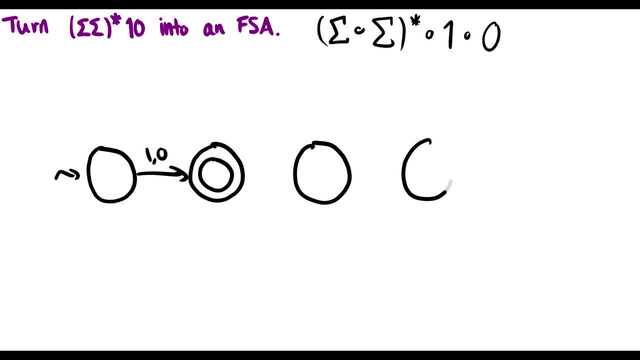 sigma, which will look like this as well. So this has another start state and this sends either 1 or 0 to the final state. Okay, so I'll do those ones in black, I will do the 1 in blue, So what? 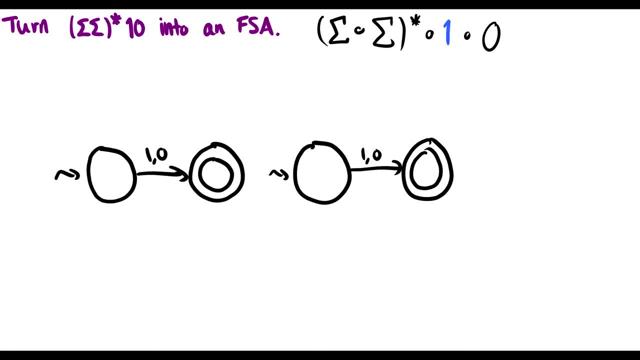 does the 1 do? It's going to send 1 to the end state. So this is going to send 1 or 0 to the end state. Okay, so I'll do those ones in black. I will do the 1 in blue. So what does the 1 do? 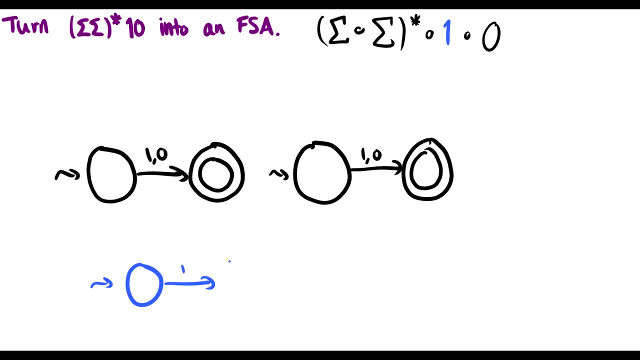 Well, we have a start state for the 1,, we send it to the end state if it's a 1, and then, finally, the 0- I'll do in green- And the 0. again, we have a start state and it sends it to the final state. So here's how we start all of these problems, And then we just 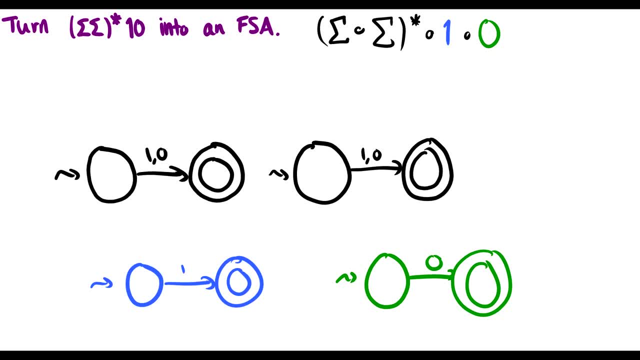 use our knowledge of operations on finite state machines and we construct the final machine. Okay, so the concatenate operator on the sigmas. So I'll do this with the orange color. We take away the final state, We take away the second start state. 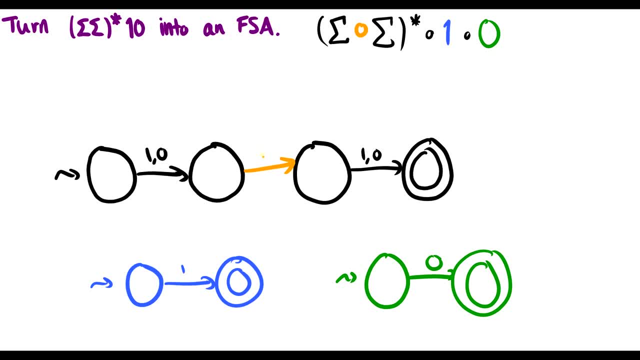 and we send the first final state to the second start state with the empty string. So now we have sigma concatenated with sigma. Now we need to store it So I can do the star in pink. So how do we do the star? Well, we create a new start state which also happens to be an end state. 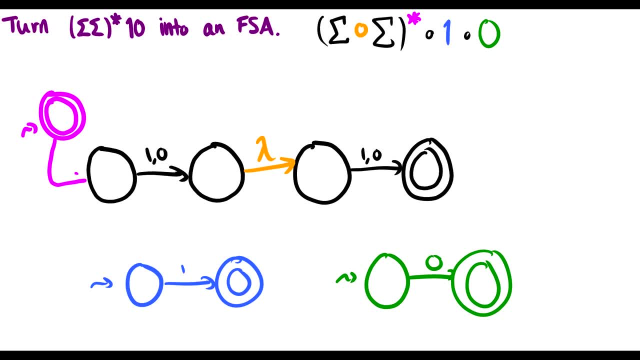 We send the new start state to the old start state with the empty string and then we loop the end state with the old start state with the empty string. So now we have sigma concatenated with sigma star. Okay, so now we need to concatenate that with one, which I will do with dark blue.